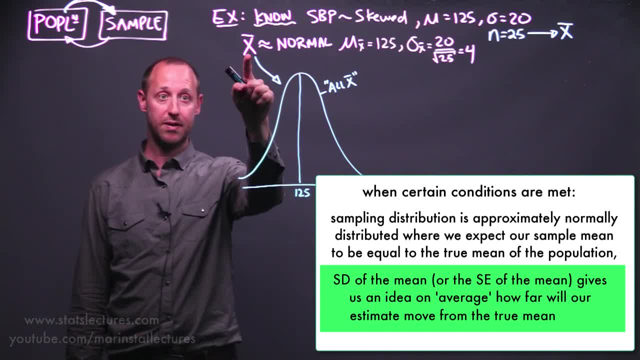 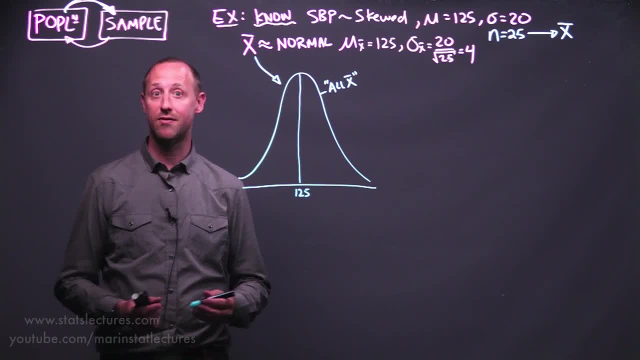 gives us an idea of, on average, how far will our estimate move from the true mean, And we worked this out to be four. So we've also learned about the 68,, 95,, 99.7 rule. So for this video, I'm. 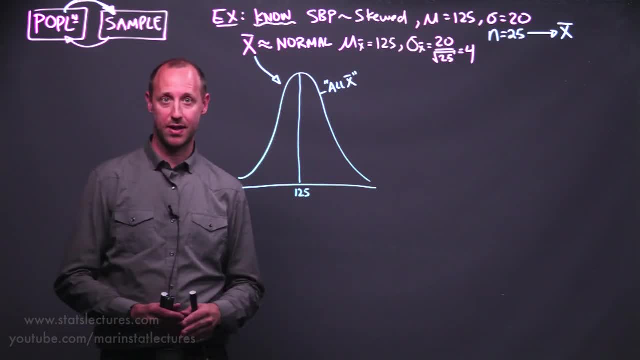 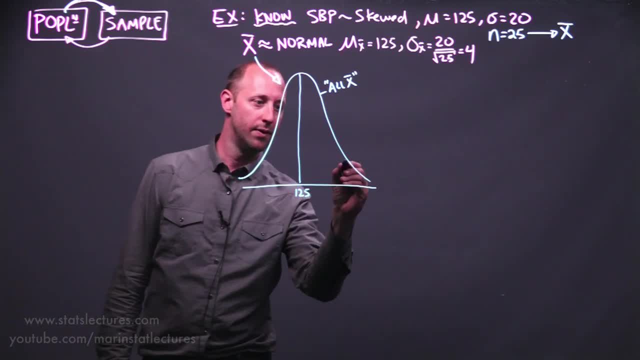 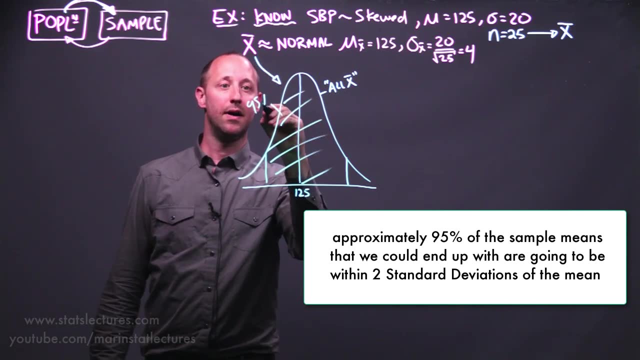 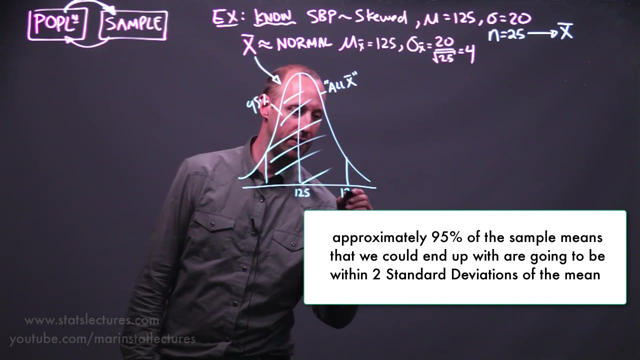 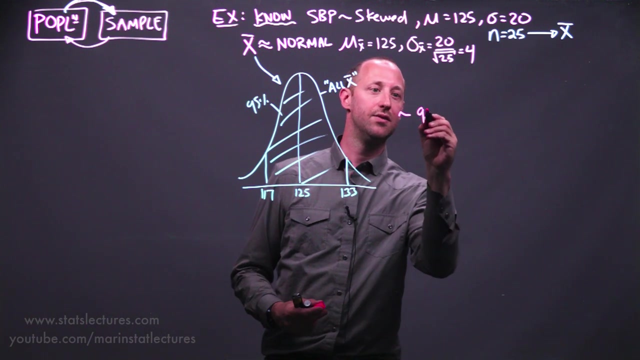 Using that two standard deviations, 95% rule, we know that approximately 95% of the sample means we could end up with are going to be within two standard deviations of the mean, or between 133 and 117.. What we know here is roughly 95% of the time. 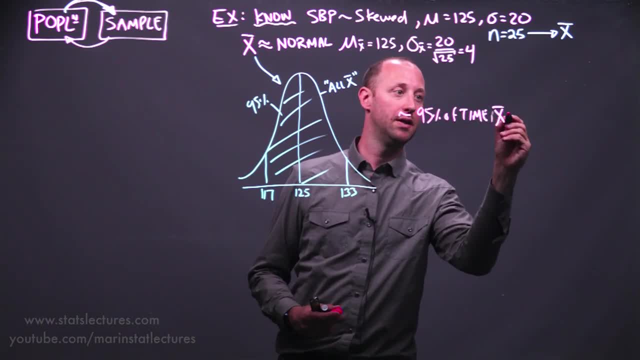 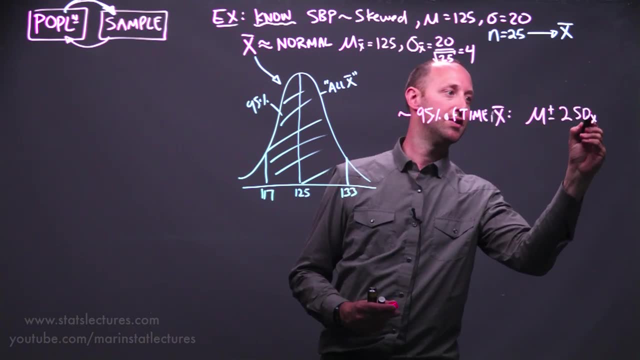 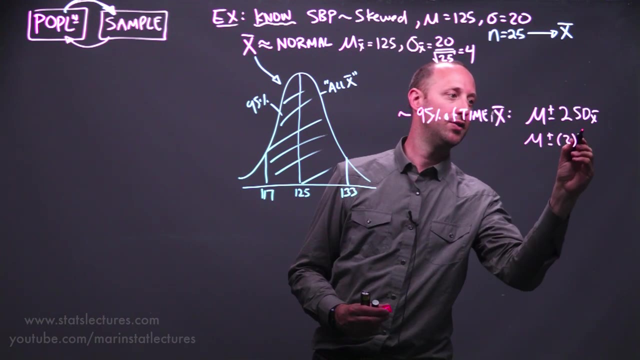 we're going to get a sample mean that is within plus or minus two standard deviations of the mean, or go from the mean plus or minus roughly two standard deviations of the mean. 95% of the sample means we can get will be in this interval here. 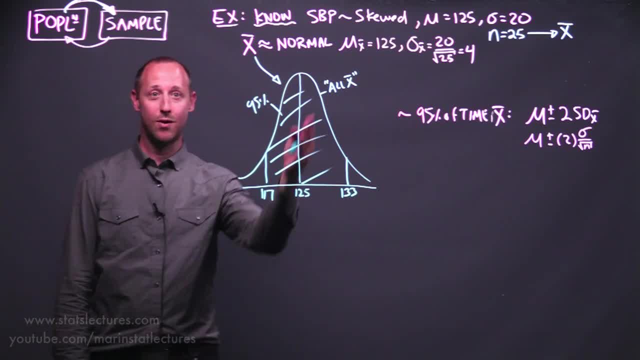 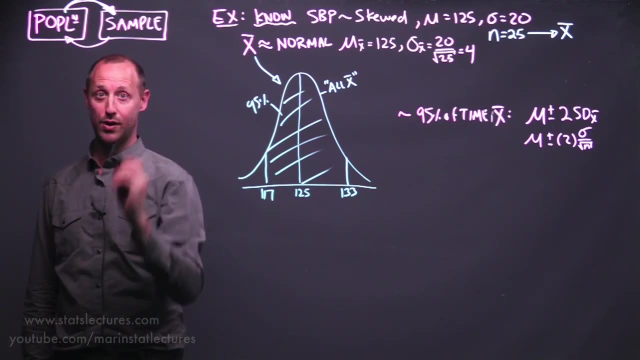 So you might be thinking at the moment: well, who cares? We never really know the true distribution, true mean or standard deviation for a population And we're not really interested in how likely a certain sample estimates will show up when we do know the truth. We're usually living in this world where we don't know the truth. 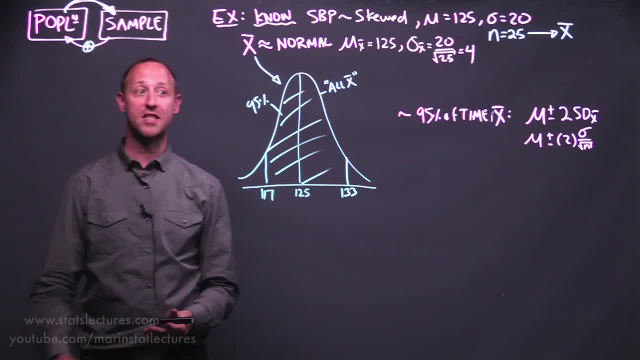 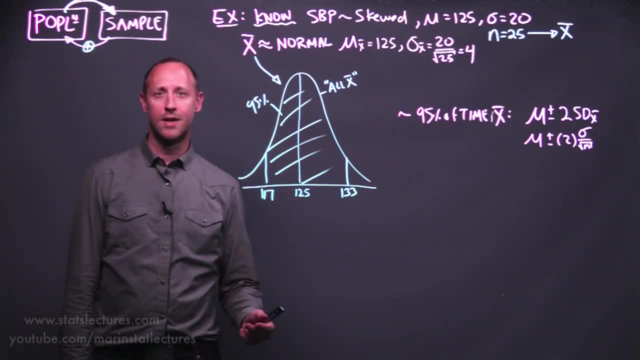 We have to collect a sample of data and we're going to use that to try and make statements about the population. But this is actually going to be very useful And we can think about it this way- If 95% of the time I'm within two meters of you. 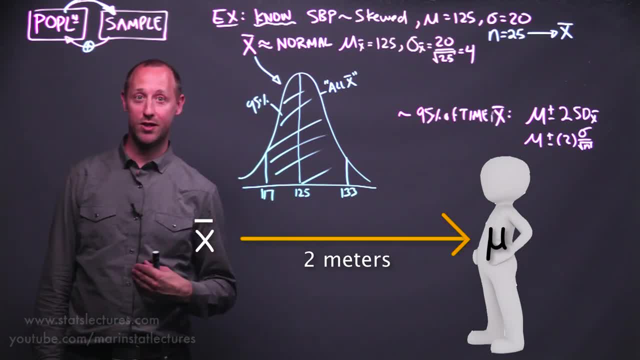 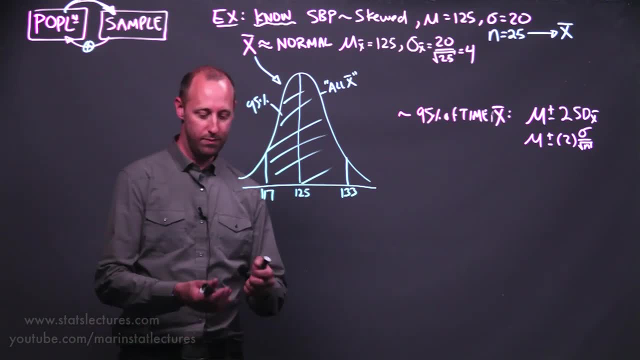 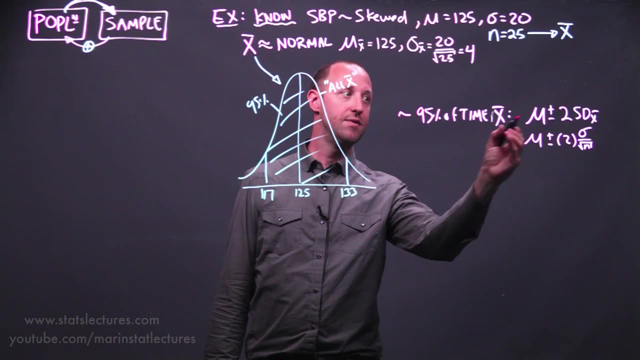 you, then 95% of the time you're going to be within 2 meters of me. The distance between A and B is the same as the distance between B and A, So we can just change our reference point here. We can say if 95% of the time the sample mean we get is going to be within, 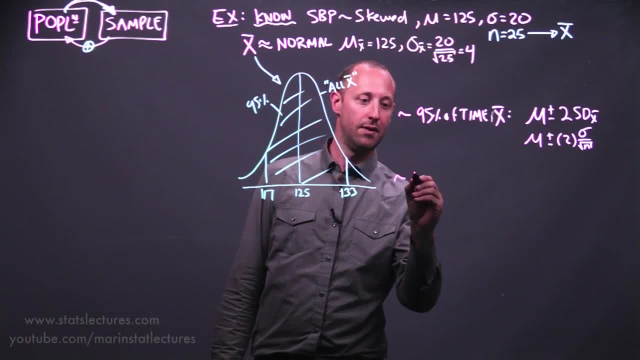 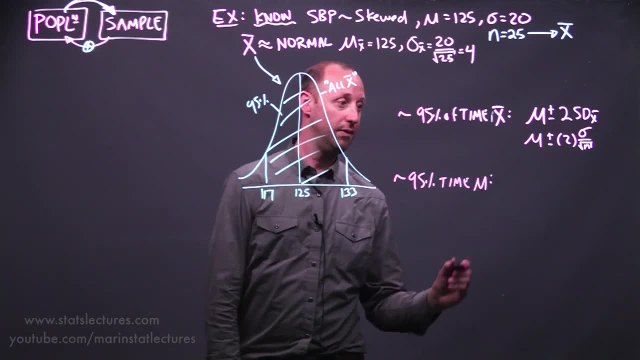 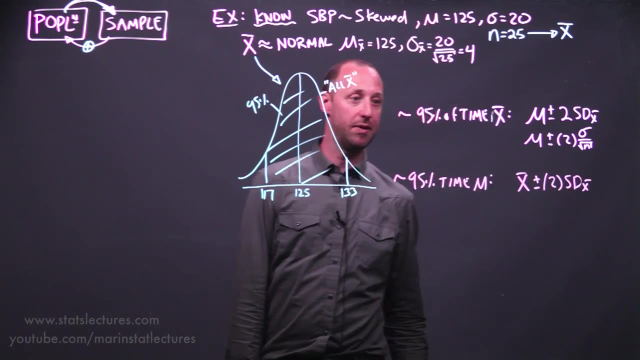 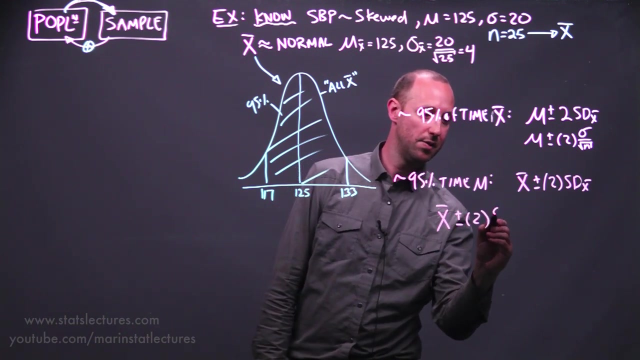 about 2 standard deviations of the true mean, then we know that roughly 95% of the time the true mean, or population mean, is going to be within about 2 standard deviations of the estimate. Or we can go from our estimate- reach out roughly 2 standard deviations of. 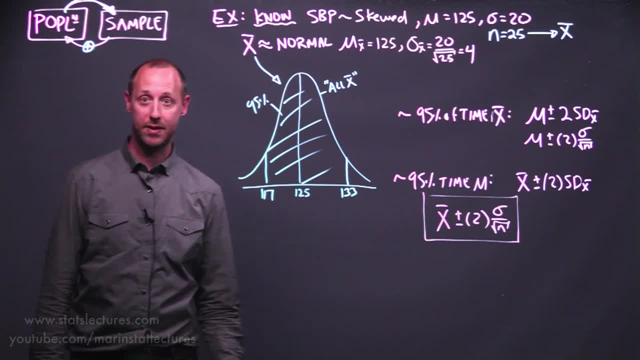 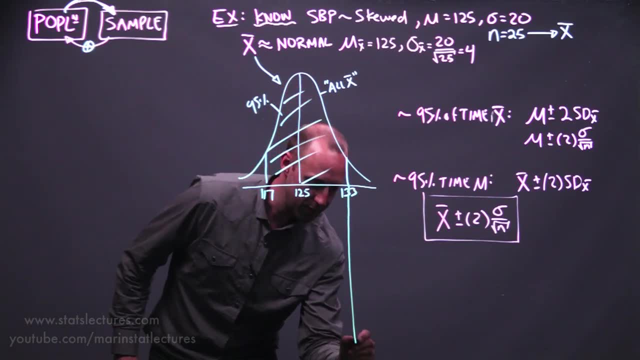 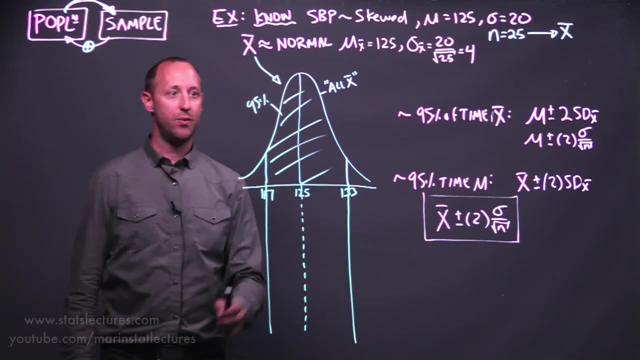 the mean. 95% of the time the true mean is going to end up in this interval. Let's take a look at this concept visually. So let's extend these downward So we can think when we reach into this population. randomly select 25 observations and calculate. 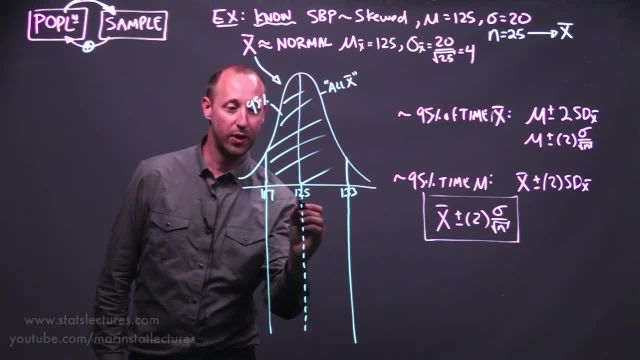 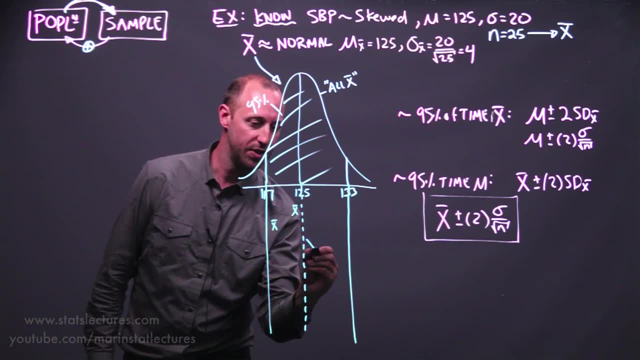 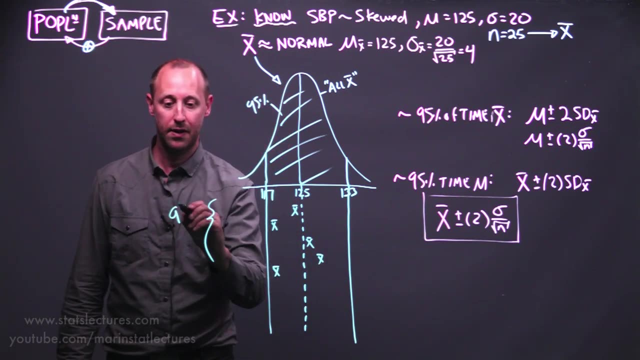 a sample mean. 95% of the time we're going to get a sample mean that stays within this interval. Maybe it's pretty close to the true mean, maybe it's a little bit further away, But 95% of the time we're going to get a sample mean that stays within this interval. 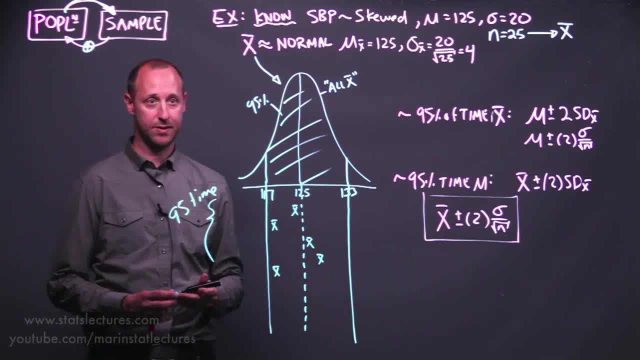 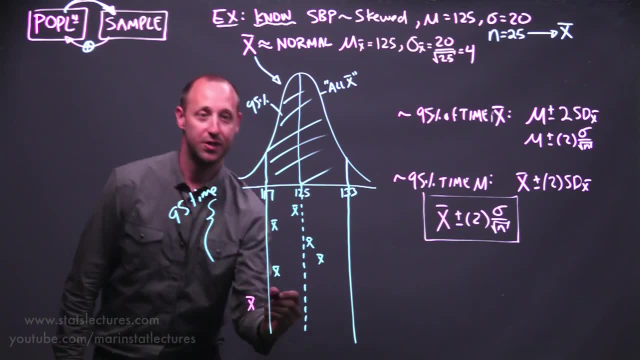 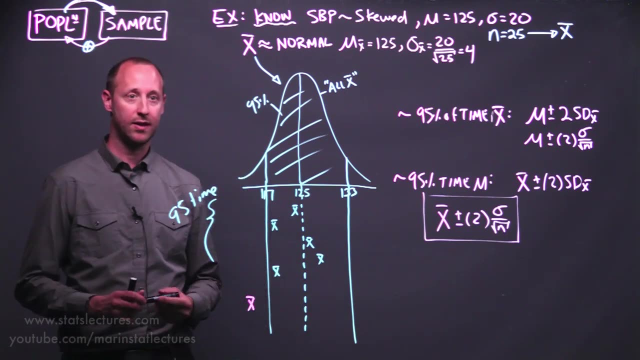 But 95% of the time we're going to get an estimate within these bounds. 5% of the time we're going to get an estimate that reaches outside of these bounds. In reality, we don't know which data, which sample we've ended up with, But we know if we go from this estimate. 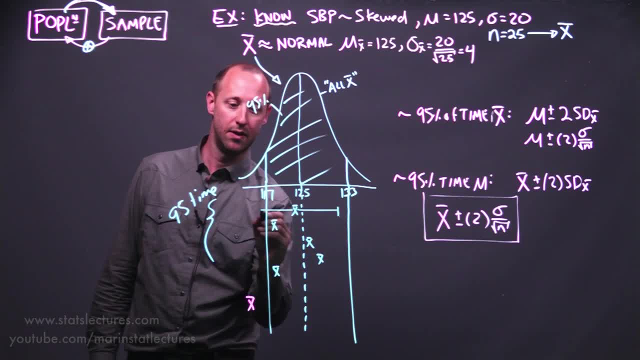 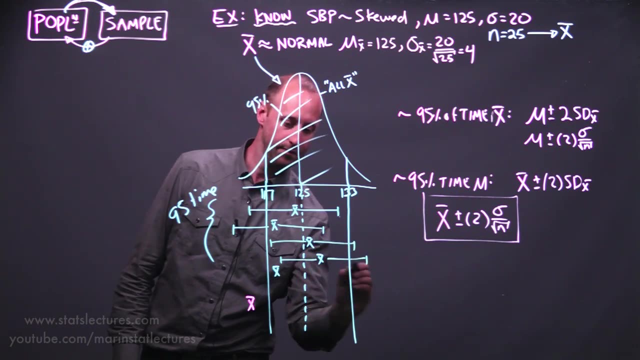 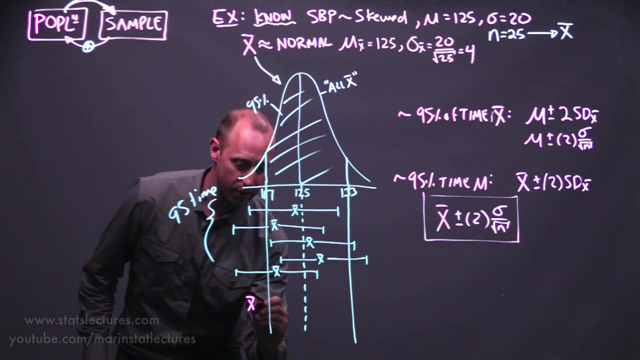 and reach out plus 2 standard deviations of the mean, minus 2 standard deviations of the mean, It overlaps with the true or population mean or contains it. Similar to this one here. For this one here, if we go and reach out 2 standard deviations above and below the, 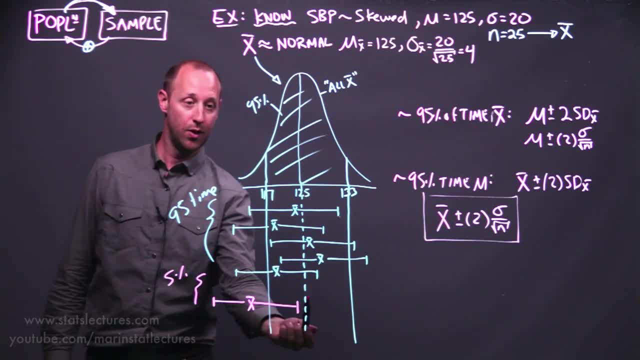 mean and these we're going to end up with 5% of the time. we can see this interval here is not going to contain the population mean. So in a real world, it's not going to contain the population mean. So in a real world, it's going to contain the population mean. 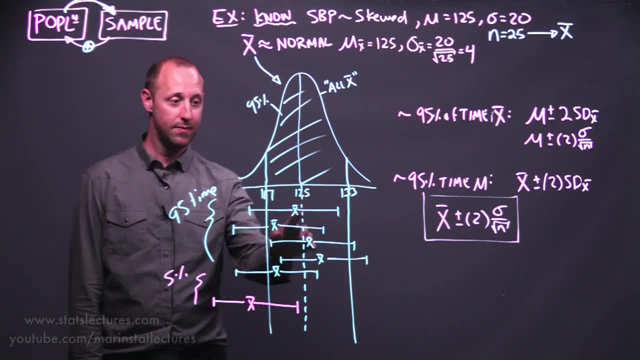 So in a real world, we only end up with one of these samples, and it either contains the population mean in there or it doesn't, But 95% of the time, our interval will. There's a few things that we're going to need to tighten up about this, and we'll start. 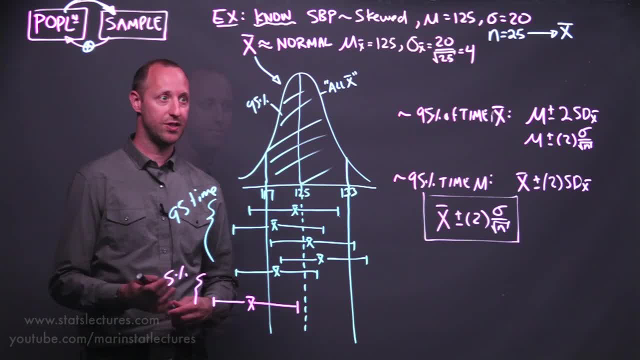 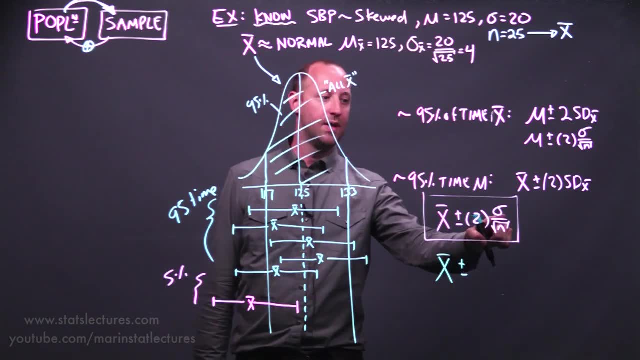 to do that in a following video when we talk more formally about confidence intervals. So a few things we're going to encounter there. The first one: you may be thinking when we're taking a sample of data and living in the world of using a sample. 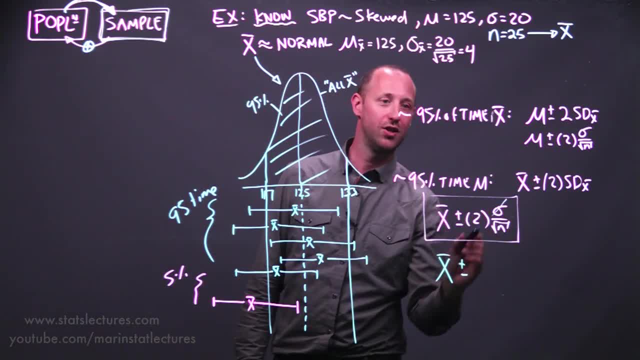 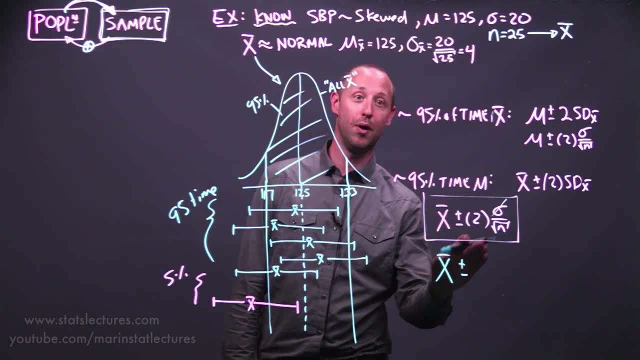 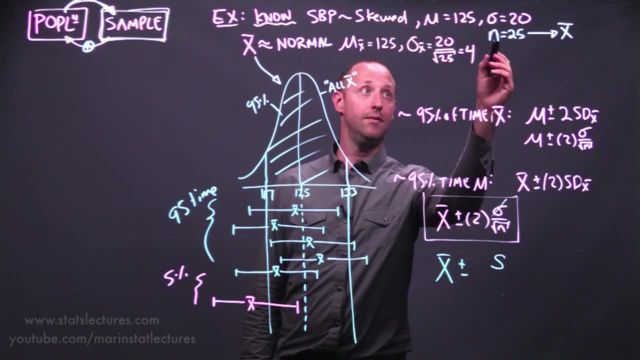 We're trying to generalize back to a population, We're not actually going to know the true standard deviation. It's difficult to imagine a scenario where we're trying to estimate a population's mean, but we know their standard deviation, So we're going to have to replace that with the sample standard deviation. 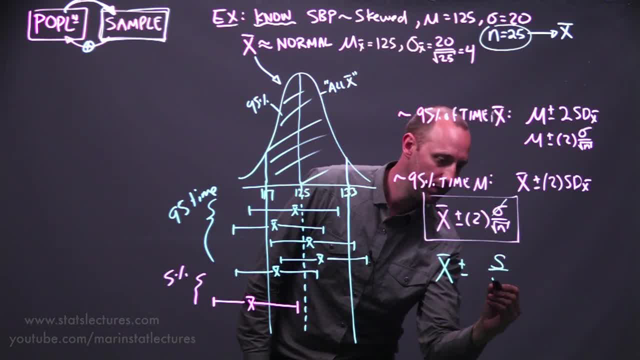 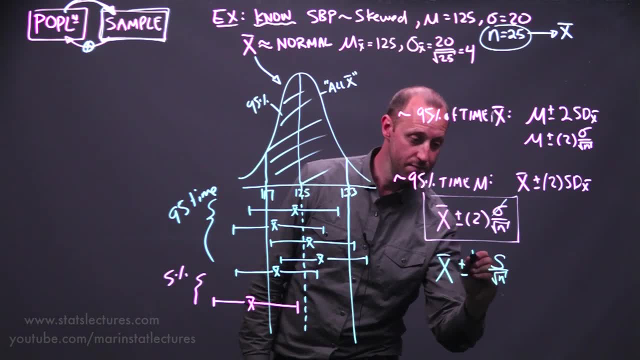 The standard deviation of our 25 observations, And that's what we're going to start to call this standard deviation of the mean, the standard error of the mean. Because of that, Rather than using z- a standard normal of 2, we're going to have to use a t value. 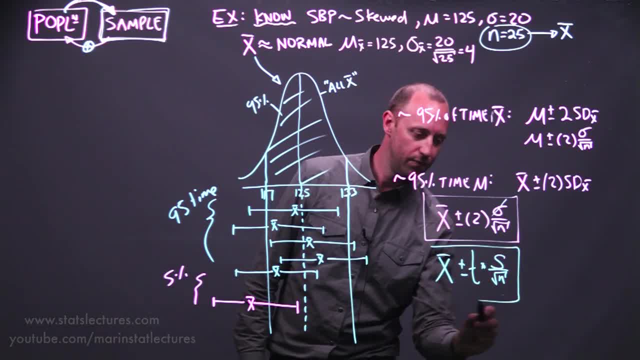 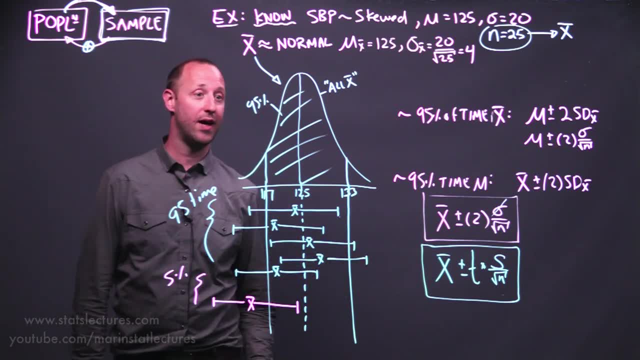 And it's going to be something slightly larger than 2.. We'll get to all those finer details when we start talking more formally about confidence intervals, But it's important to note that all the concepts we've talked about hold, And that's why we've left out this discussion for now. 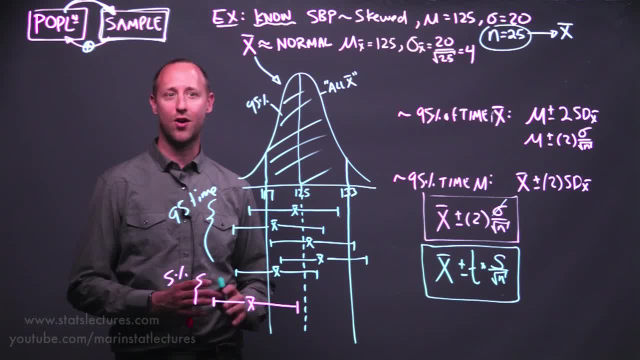 If we start to talk about the t distribution and all these things, it clouds the concept of what is a confidence interval actually trying to achieve And what are the concepts it's based on. One final thing: We'll talk about this more in the next video. 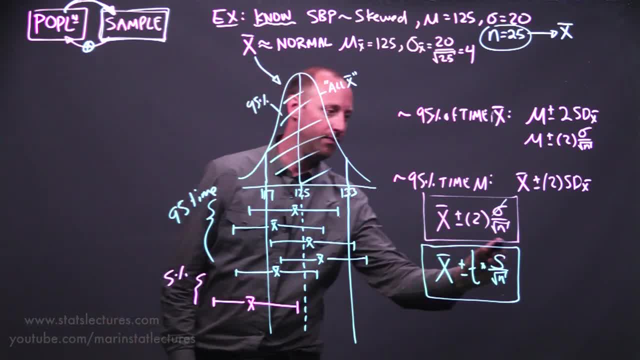 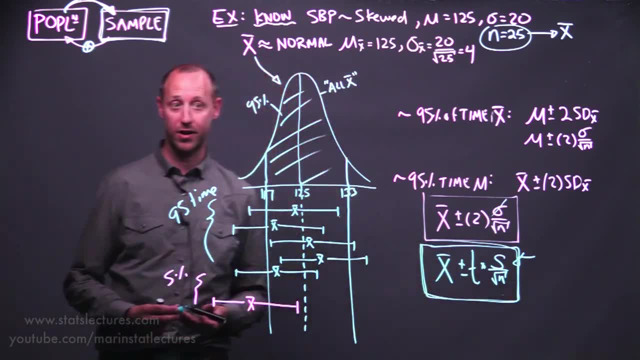 But when we build these confidence intervals we don't end up saying there's a 95% chance that the true or population mean is contained in our interval. We're going to say we're 95% confident it's in there. And the reason being- and we'll expand on this later- in a real world we end up with: 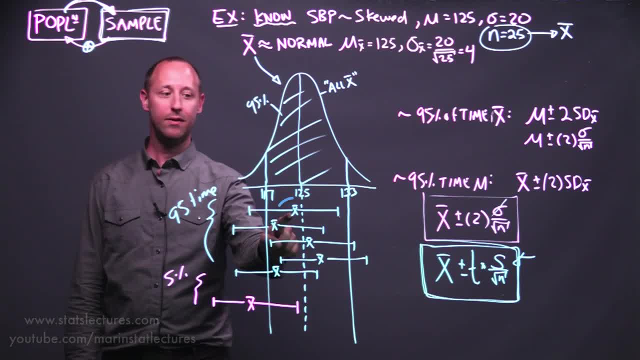 one of these samples of data Now looking at this blue one here. There's a blue one here. There's not a 95% chance the population mean's in there, It's 100%, It is in there. Taking out this one here, and what's the chance that the true or population mean is in this? 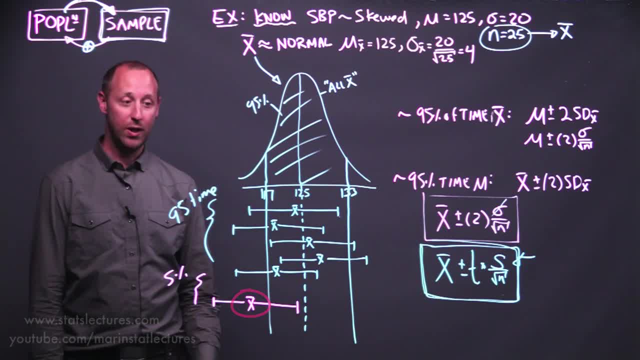 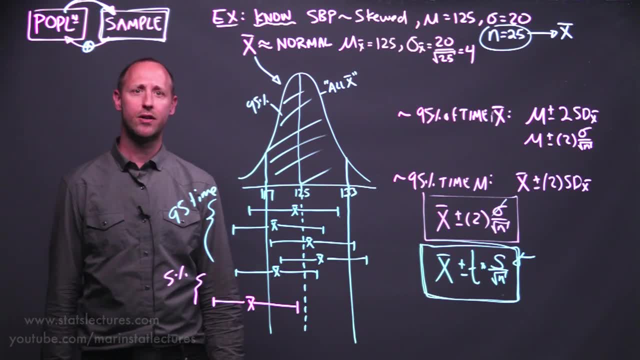 interval Zero. It's not contained in there. When we take a sample of data, we don't actually know which sample mean we've got and which interval we've got. So that's why we're going to end up saying we're 95% confident. our interval overlaps.